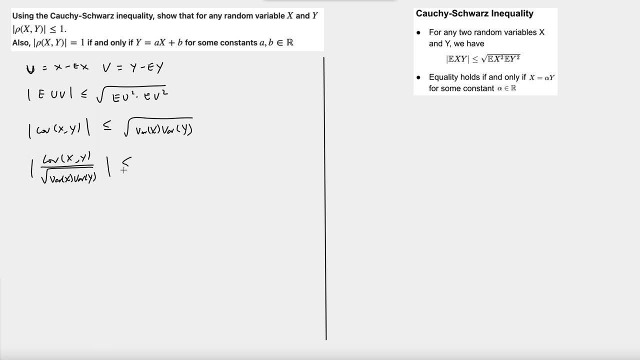 So we have the covariance of y and this is less than 1, and so this is just say this is the same as the row absolute value is less than or equal to 1, because here it's just the definition of row, right. So the second question: the absolute value of a row is 1 if, and only if, y is equal to a, x plus b, for some constant a and b. 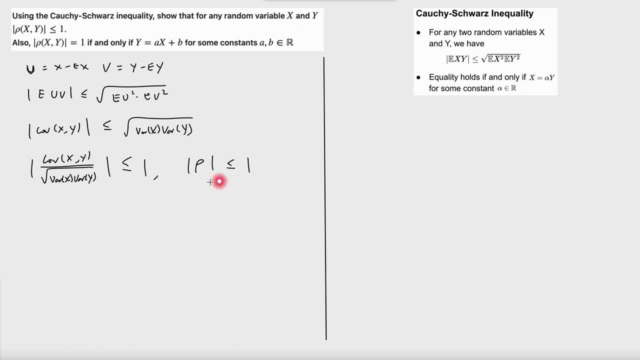 So now, first row is equal to 1.. The absolute value of a row equal to 1. It means that the equality holds here, and means equality holds here, and if the equality holds here, and that means the equality holds here, right. So in other words, the absolute value of a row is equal to 1 means the equality holds here, right. 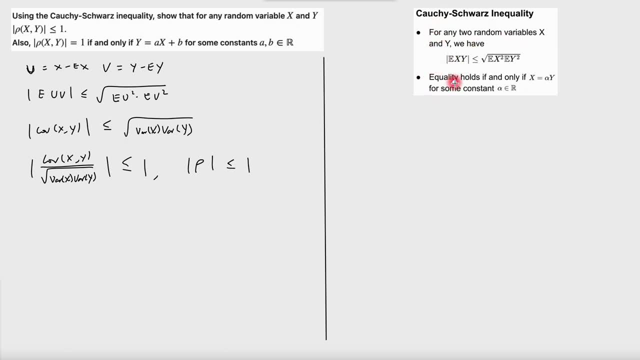 I mean, based on what we just showed here, the equality in this inequality holds if, and only if, x is equal to alpha y. We can here, we can just apply this to u and v. So we, We, We say row is equal to 1.. 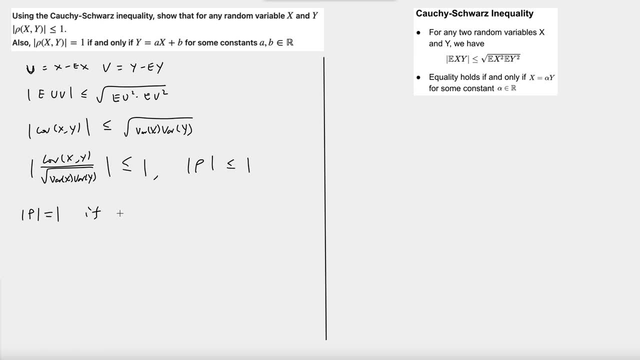 I mean the absolute value of row is equal to 1 if, and only if, v is equal to alpha u for some alpha right, And this is the same as y minus ey is equal to alpha times, x minus ex. We're not done yet because we need to show now. we show that the row absolute value of a row is equal to 1.. 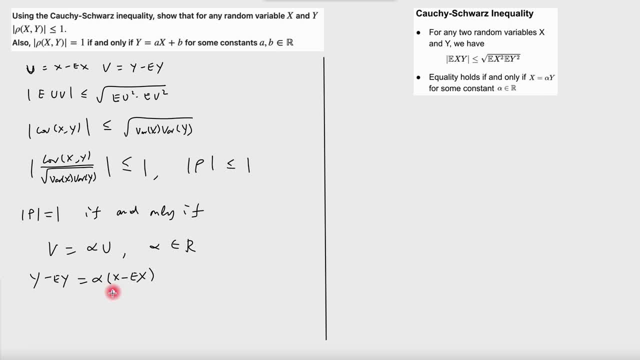 If, and only if, y minus ey is equal to alpha times x minus ex. but we still need to show that this is the same as saying y is equal to ax plus b, right? So we need to show that this is equivalent to say y is equal to ax plus b- for some a and b, right? 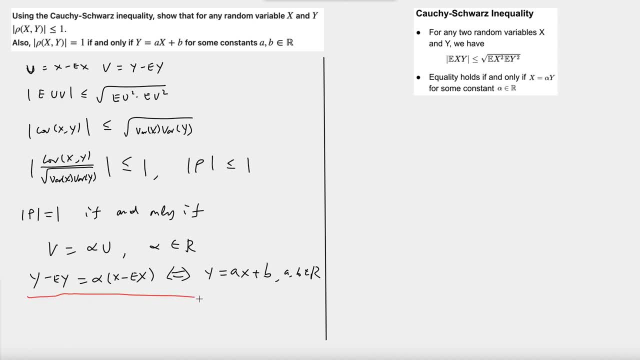 So we need to prove this statement right now. Let's first prove that the left-hand side, So we need to prove that the left-hand side implies the right-hand side, And that's- this is a pretty obvious, because the left-hand side just says that y must be equal to alpha, x plus ey minus ex right.